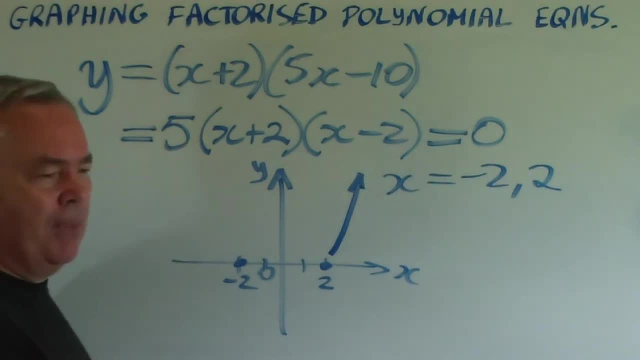 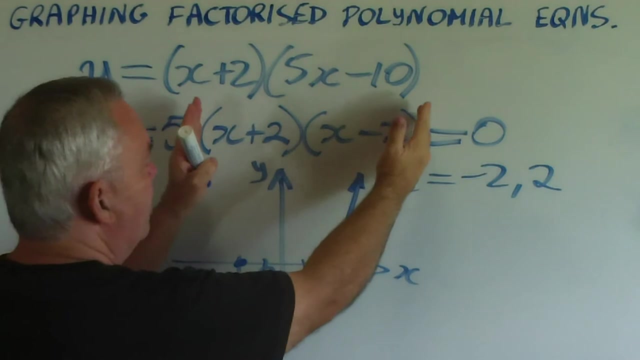 What does a number, a leading coefficient of 5 or 10 or 15 or 18 do to a polynomial? Well, the simple fact is that it means that the y value gets much, much larger, Whatever this product is worth, 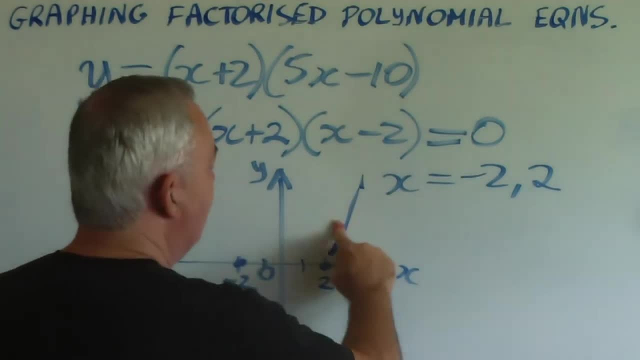 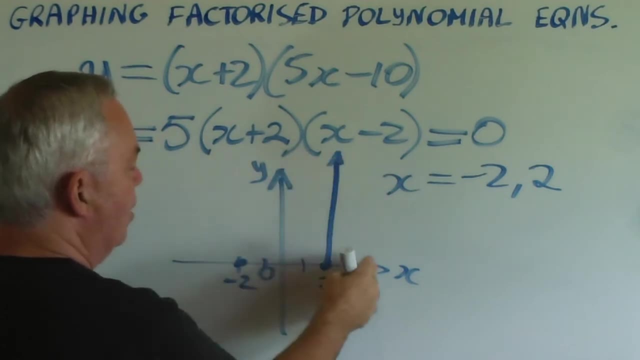 we have to multiply it by 5. And it has the effect of making the graph very much deeper. For a small increase in x, we get a very much larger increase in y. So this parabola, in fact, and this is going to disappear from your video- 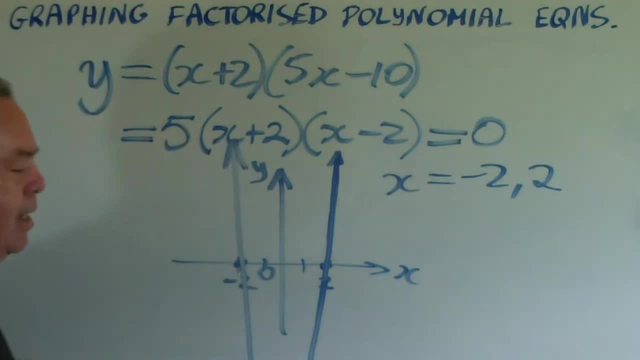 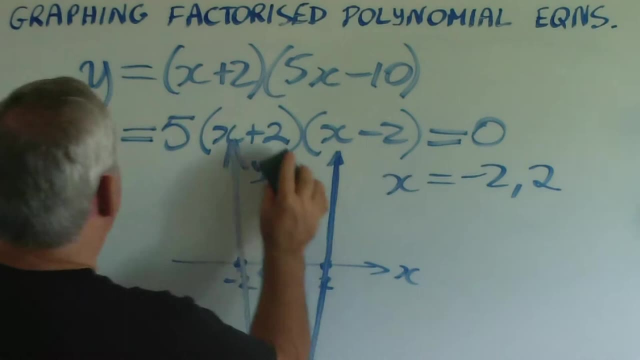 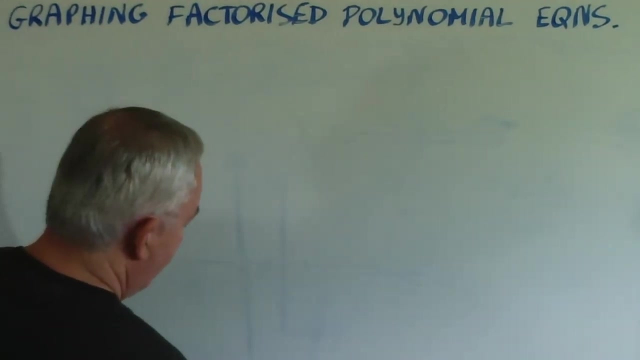 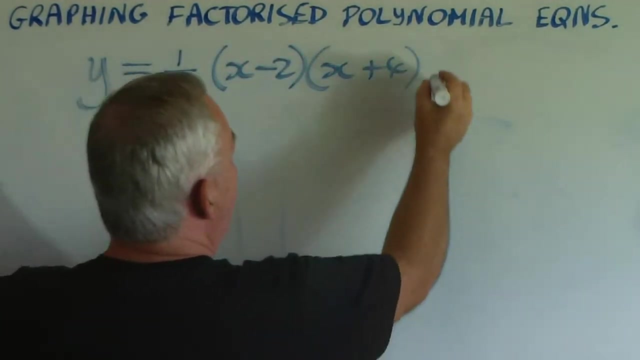 would go way down below the axis. What would be the effect of having a small factor? Well, let's check that out. What if we had something like 1 half x minus 2 x plus 4?? Again finding the roots. 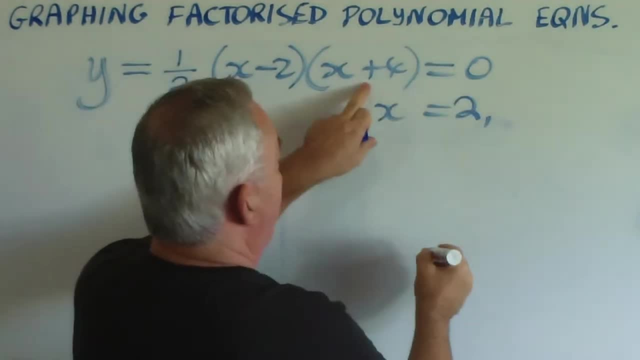 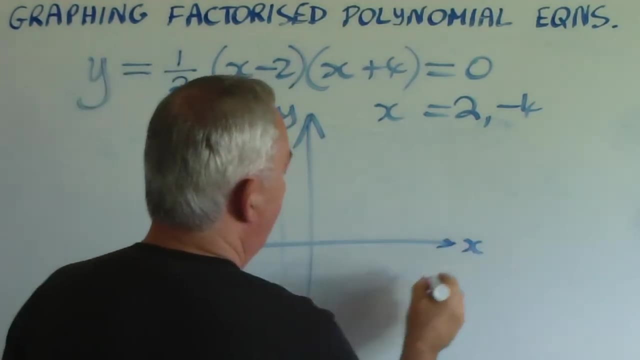 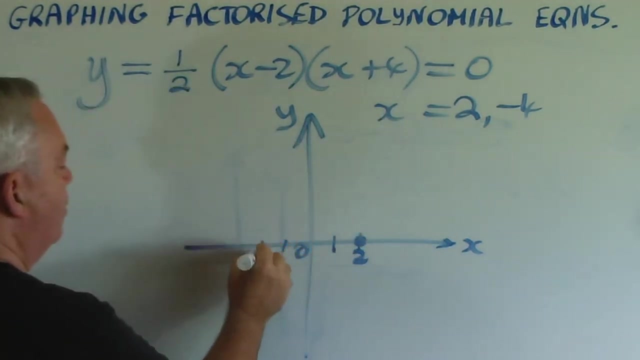 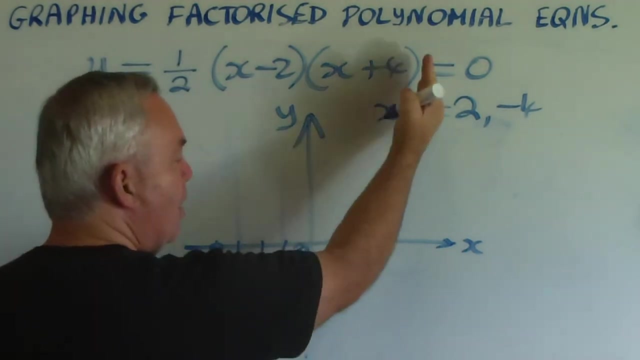 there'll be a root at x equals 2, and a root at negative 4.. Let's plot the roots: 2, negative 4.. It's a positive value. so we know the graph is rising as x increases, but it's only a half. 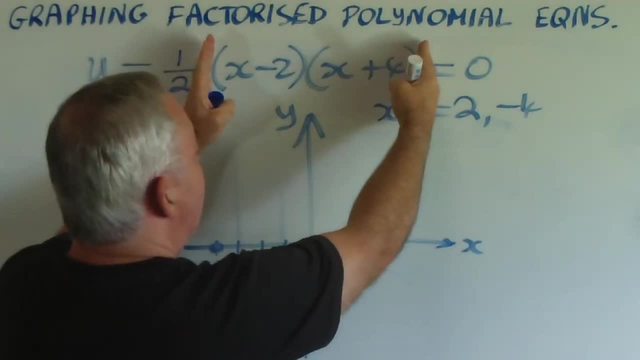 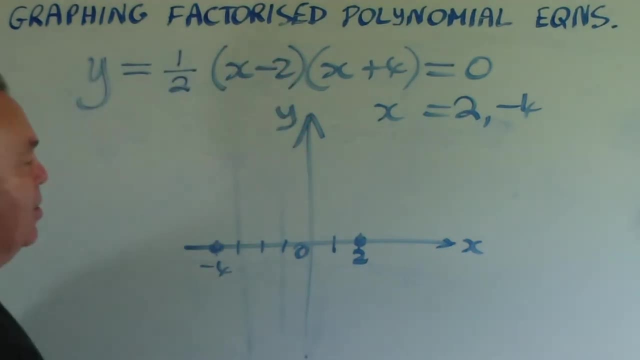 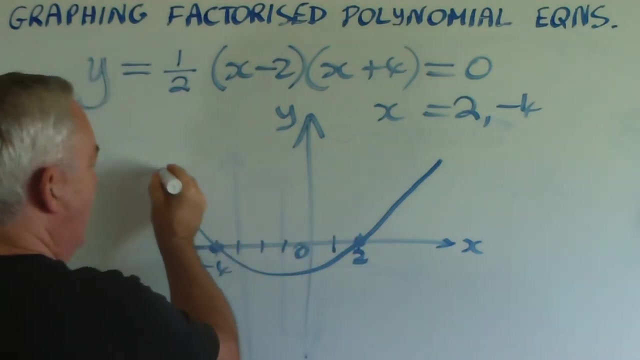 It means that whatever value this expression takes, we halve it before we find the y value, And that has the effect of shrinking the y axis. So instead of being a relatively steep parabola, it now is rather flattened. I don't think I did a good job of that. 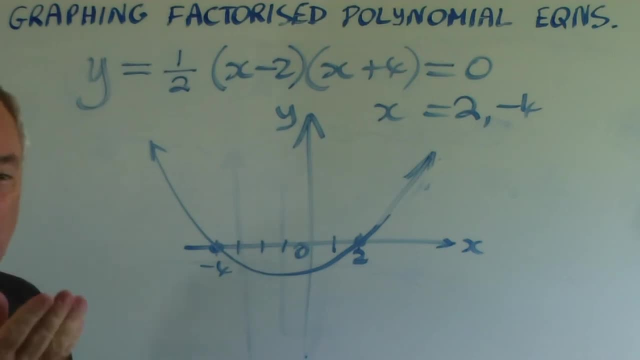 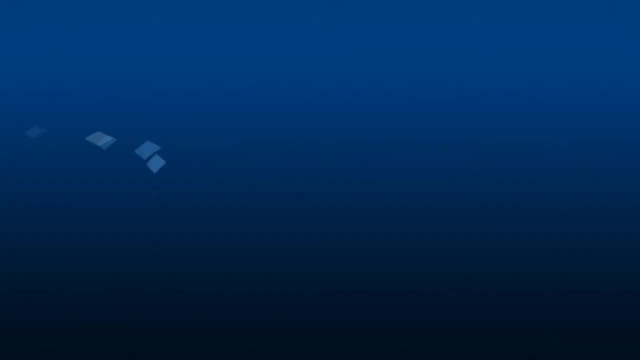 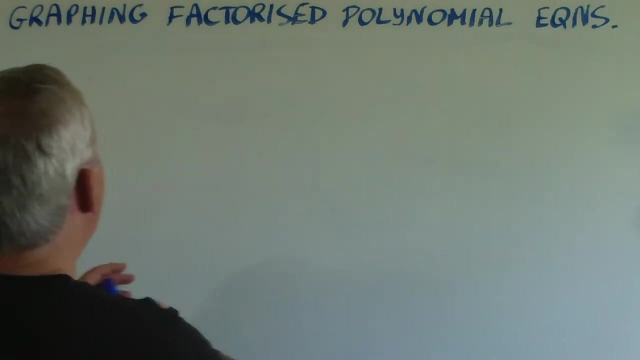 So leading coefficients are worth studying because they tell you the steepness of a graph. Let's apply it to a straight line. I'm going to choose a fairly simple line and we can consider this as a polynomial with one factor. Notice, the coefficient of x is 2,. 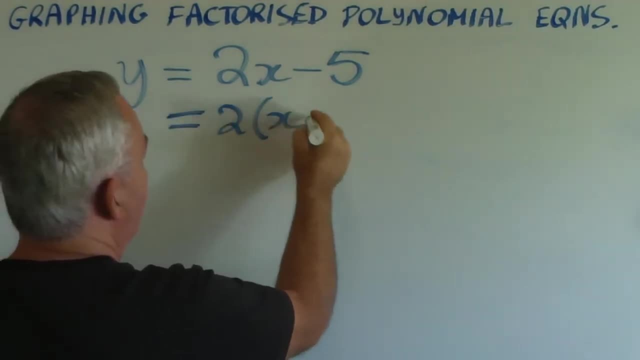 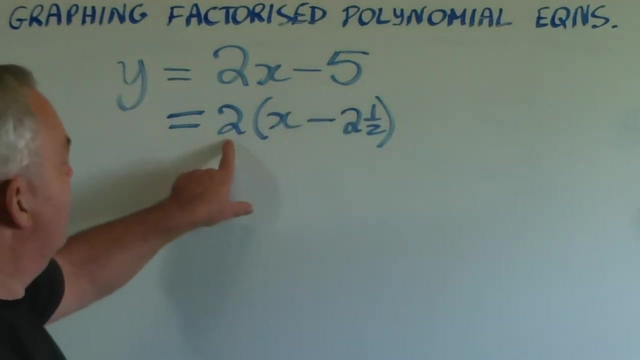 and we can remove that as a common factor. Now, 2 into 5 goes 2 and a half times or 2.5 times. so 2 times x is 2x, and 2 times minus 2 and a half is minus 5.. 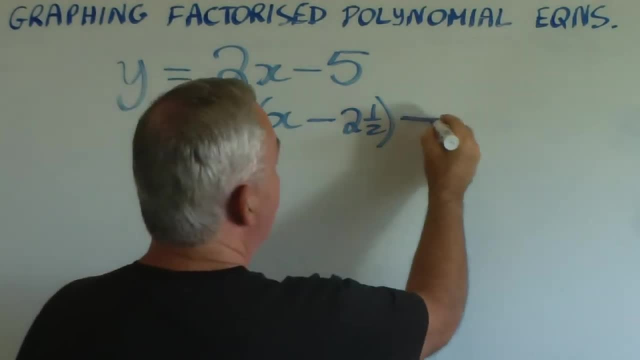 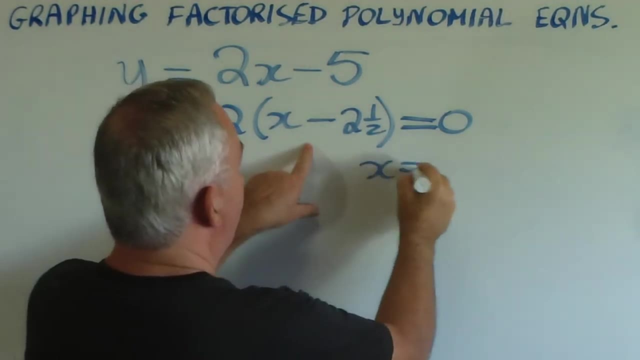 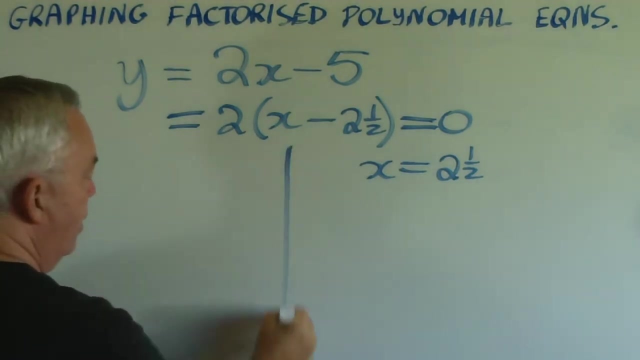 And this is the factorization that we would like, Again, to find the root of this polynomial. we set y equal to 0, and we find there's a root when x is worth 2 and a half. So, as you can see, 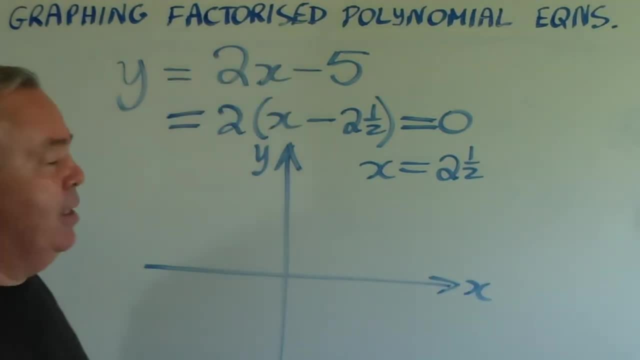 another consequence of having more complicated factors is sometimes the roots are not whole numbers. So we plot this root at 2 and a half. We know that it's a positive polynomial, or at least the leading coefficient is positive, which means that the polynomial will increase as x increases. 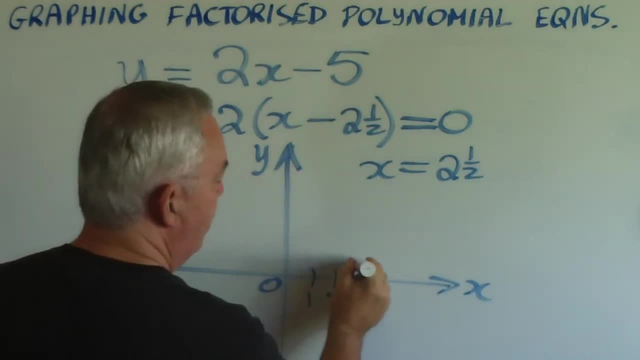 and 2 means it's steeper. So instead of going out like this, it actually is steeper. Now, in the case of lines, it's very simple. It means for every value of x you go across, you go up two squares. 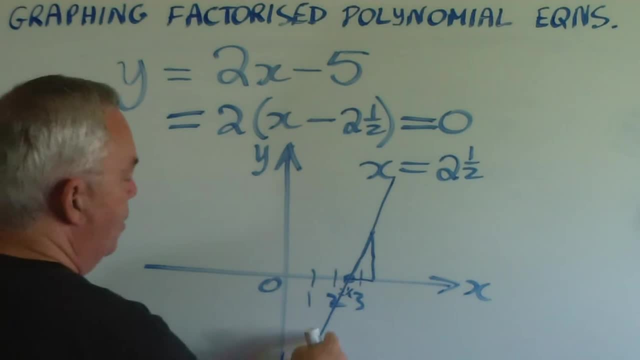 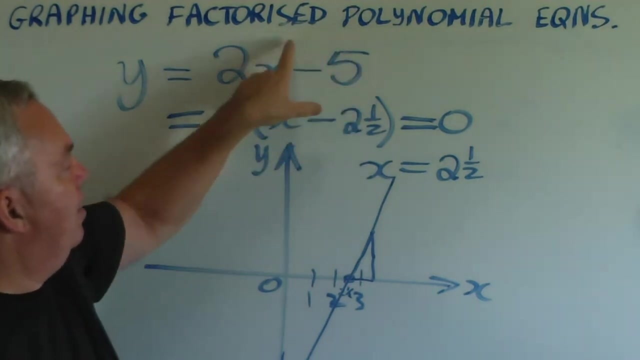 And you can see that in fact the distance along the x-axis is going to be half the distance along the y-axis. So if that's 2 and a half, this is going to be at minus 5, and of course that's the y-intercept that we can read from the equation. anyway, 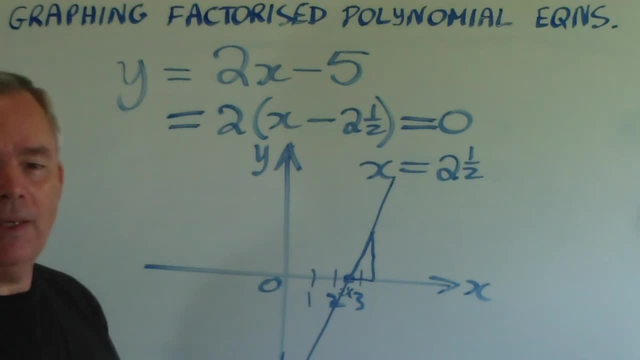 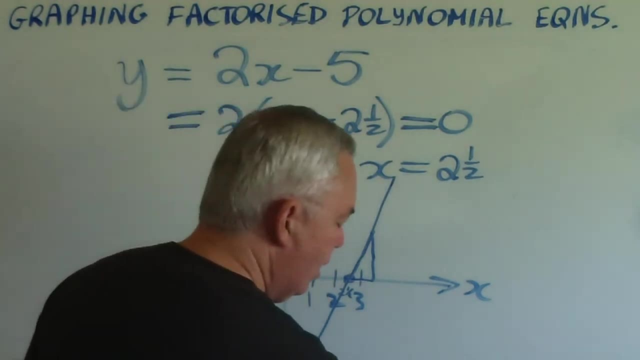 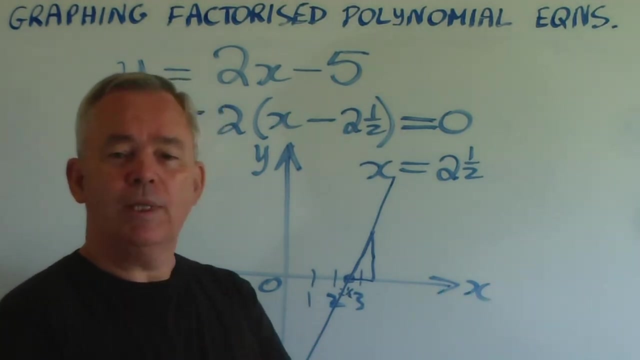 But this is just a slightly different way of looking at the equation: for a straight line to identify its root by factorizing. We're going to do one last example, and that's a slightly more complicated one, to put it all together and show that we can have. 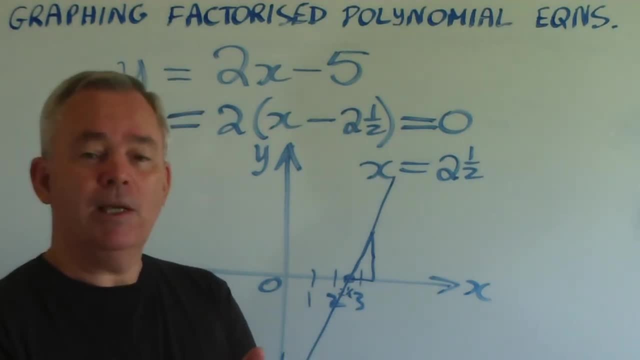 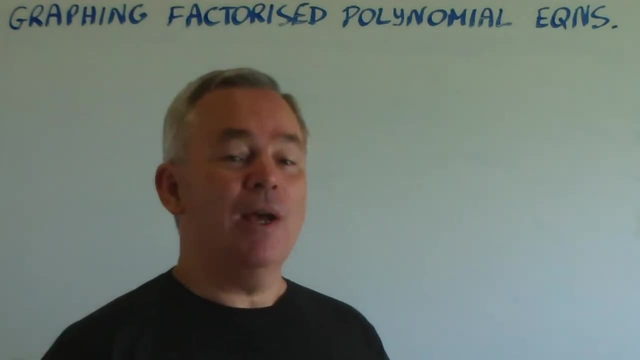 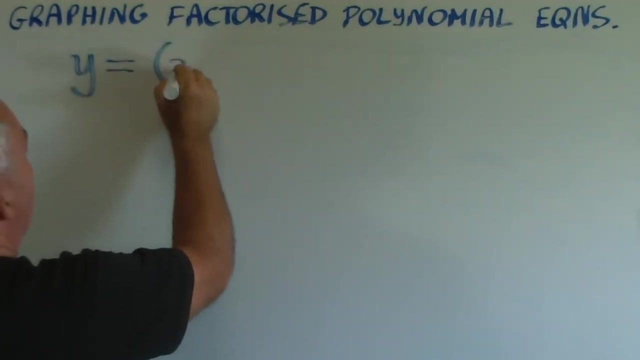 a negative large leading coefficient with roots that are not all whole numbers. So let's have a look at that. Now let's graph just one more polynomial. We're going to draw one that has a simple factor, one that has a reversed factor. 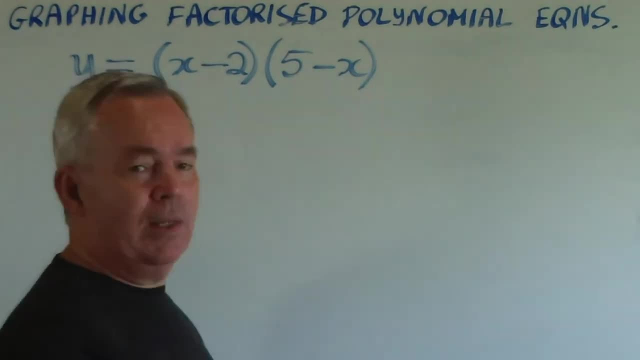 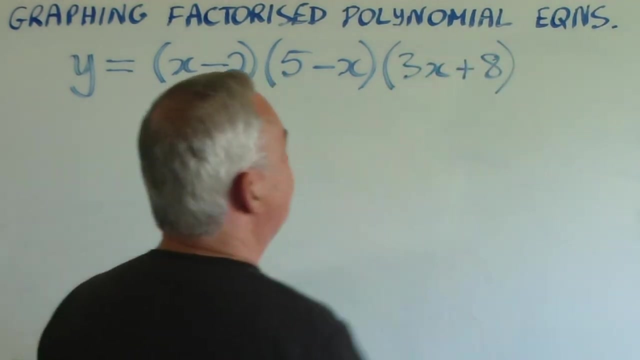 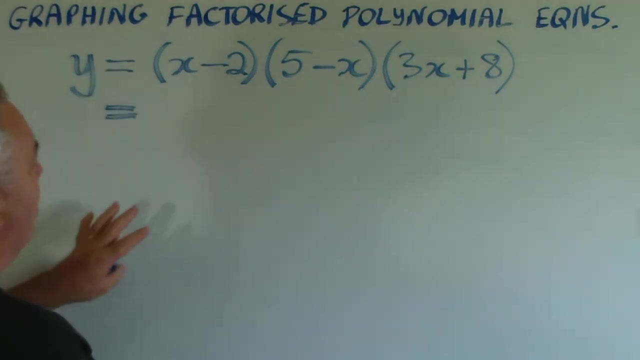 and one that has a slightly more complicated factor, And let's see the effect of putting all this together. If we fully factorize this, the first term doesn't need any change, but the second term. the coefficient of x is minus 1,. 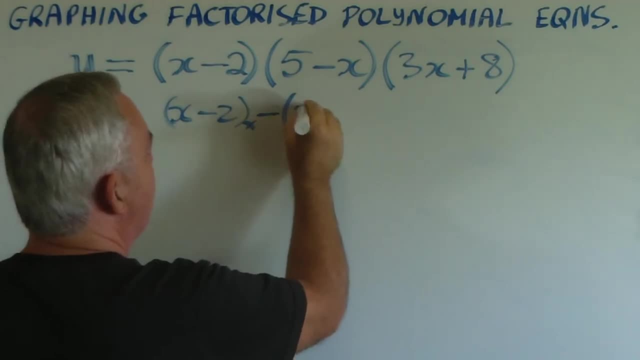 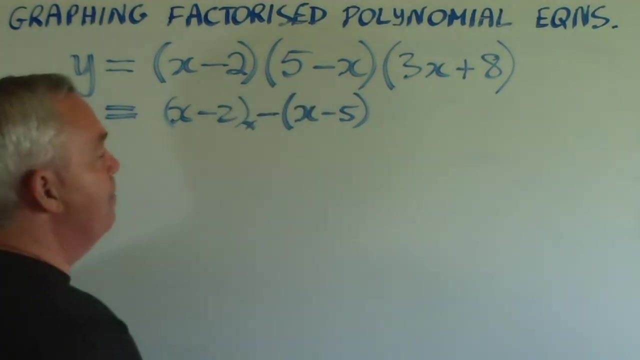 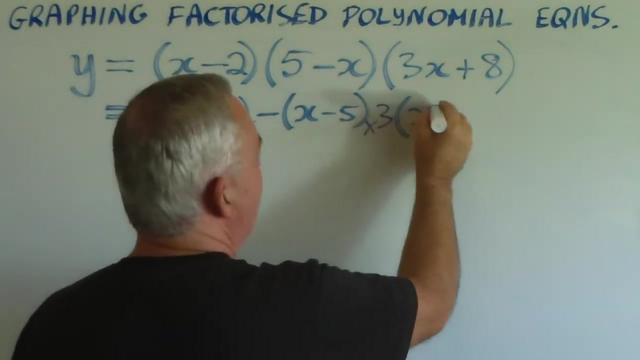 and we can take that out outside the parentheses so that minus x gives minus x and minus minus 5 gives plus 5, and here the coefficient of x is 3, and we can take that outside the parentheses and fully factorize this factor. 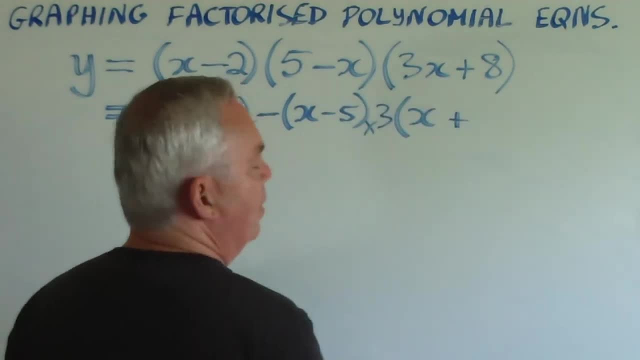 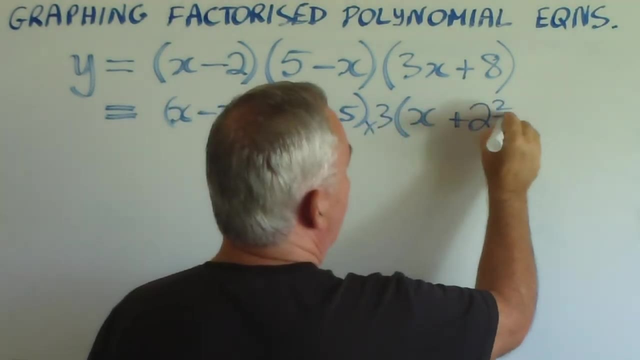 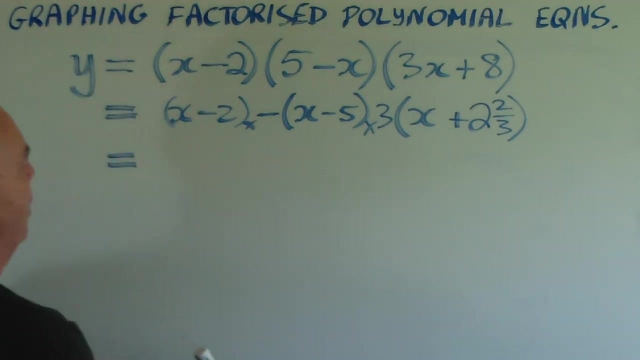 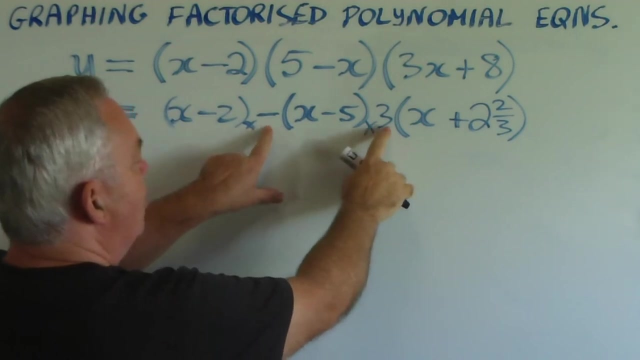 3 times x is 3x, and you'll excuse me if I use fractions rather than decimals, but 3 times 2 and 2x. 2 and 2 thirds makes 8.. We can keep these factors together, but these two constants. 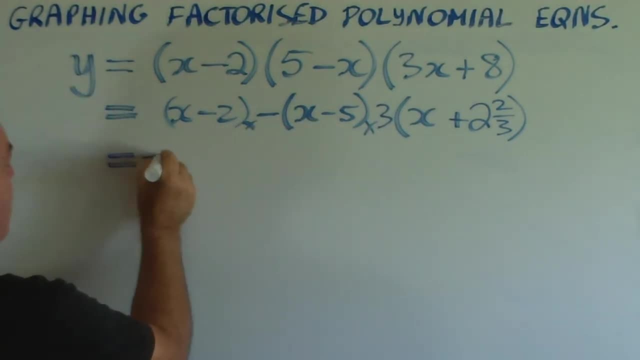 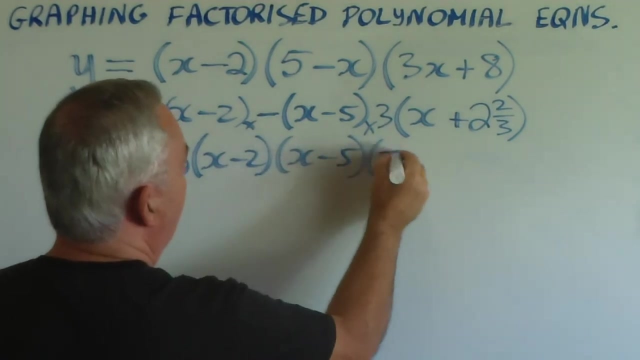 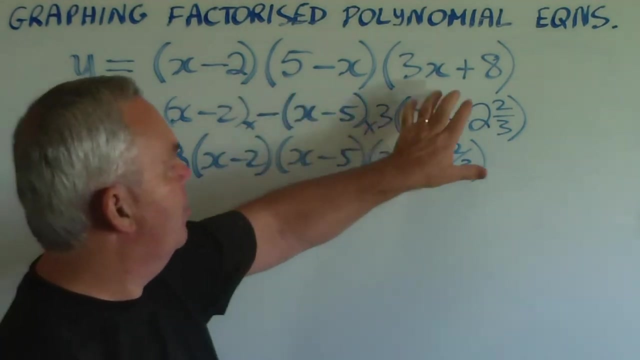 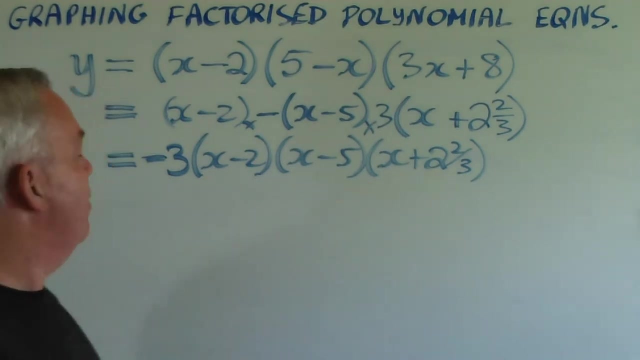 the minus 1 and the 3, we can multiply and bring out the front And straight away you can see the effect of having reversed terms and more complicated terms. That is, we sometimes get more complicated roots and we do get a leading term. 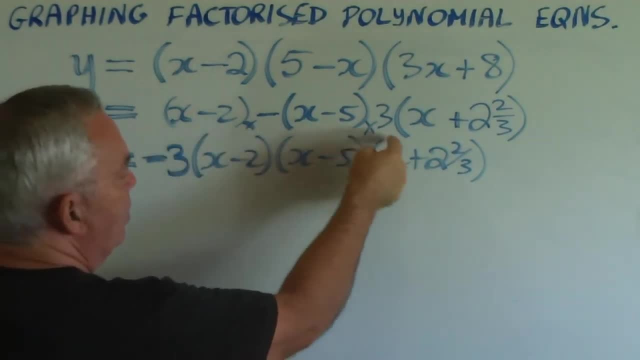 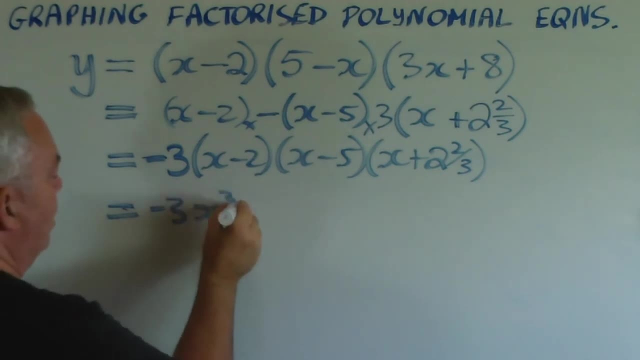 If we expanded this, we get x times x. times x would give us the x cubed and its coefficient would be minus 3, and there would be other terms. What is the effect of that minus 3?? Well, I hope you know by now. 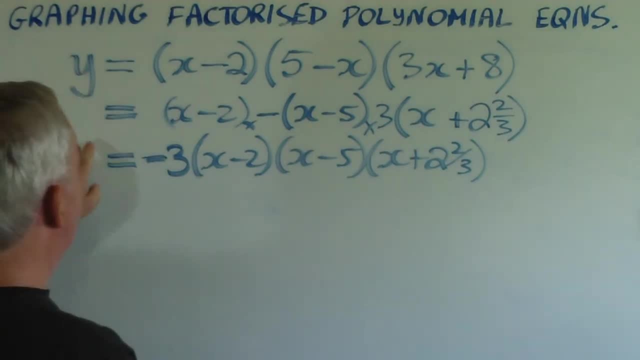 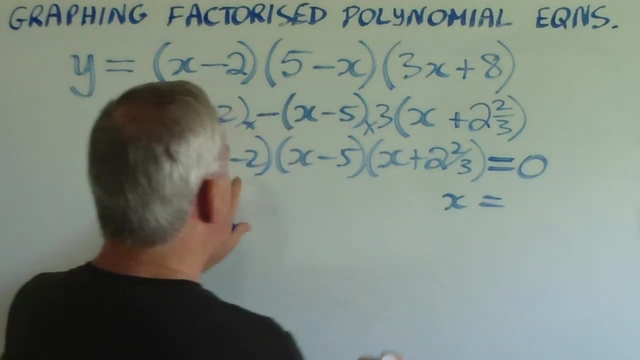 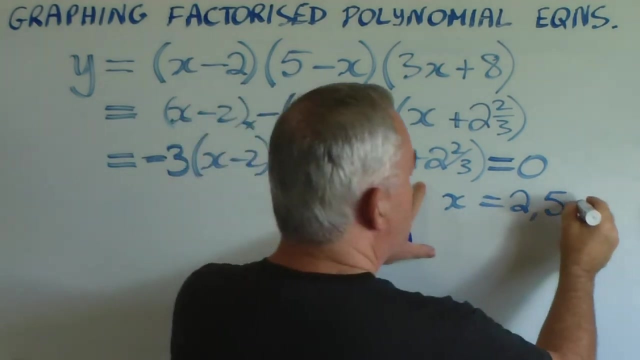 but let's draw this graph To find its roots. we set y equal to 0.. We can then determine the three roots. There will be a root at plus 2, a root at plus 5, and a root at minus 2 and 2 thirds. 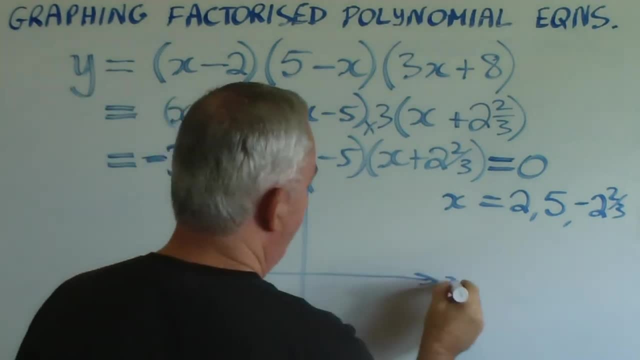 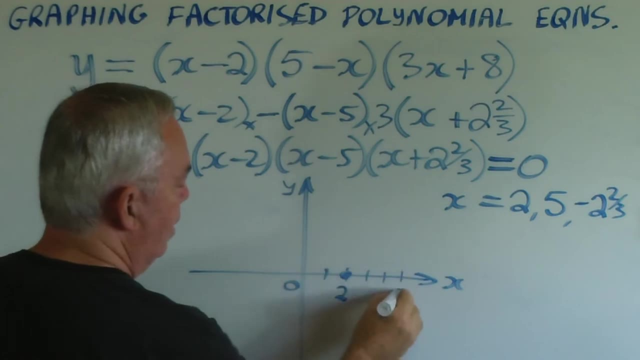 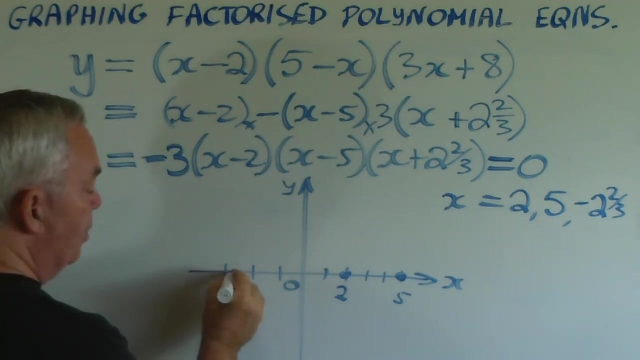 We draw the axes: One root at 2, another root at 5, minus 2 and minus 3, so minus 2 and 2 thirds will be about there, And our graph has to pass through these three roots. 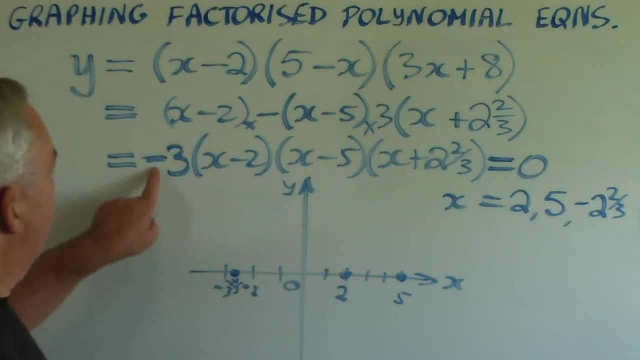 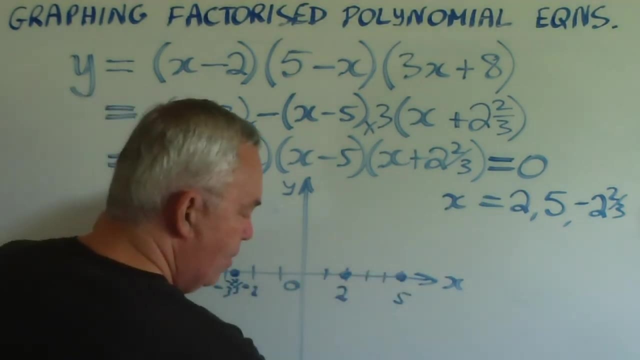 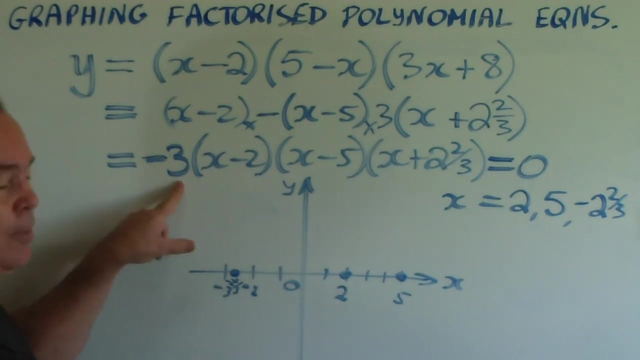 these three zeros, these three points. The leading coefficient of minus 3, the minus sign means that the graph must head downwards at the right. As x increases in value, y will increase negatively And the 3 means it will do so steeply. 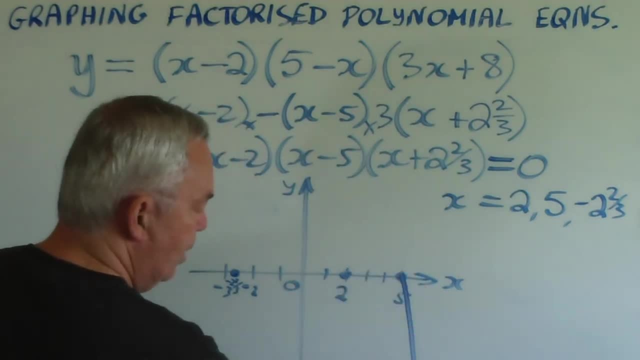 So instead of just going in a nice smooth curve, this will go down quite steeply, which means, of course, it will rise quite steeply here Now I'm going to disappear off the bottom of the video here. This will go way, way down below. 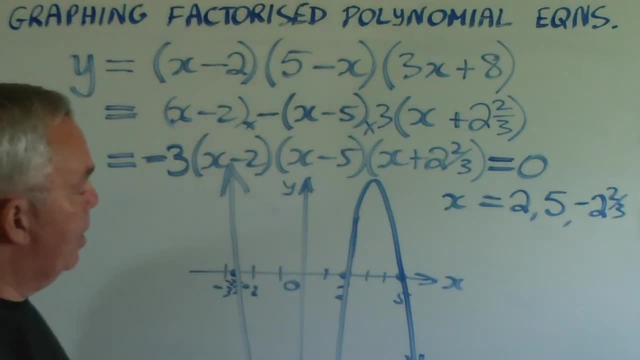 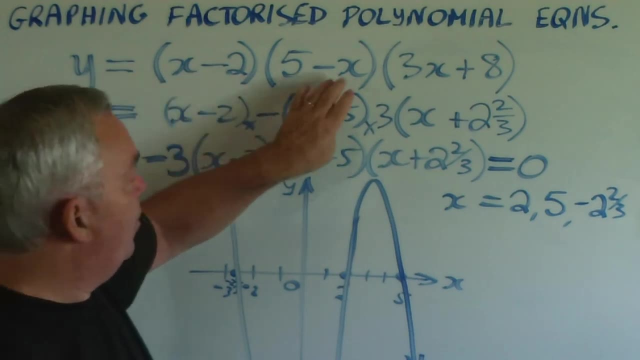 and up through here and you can see our cubic equation, a typical S shape. But there it is the effect of the first two variations on our theme, having reversed and more complicated factors. If you're very fast, you can sometimes just inspect the terms. 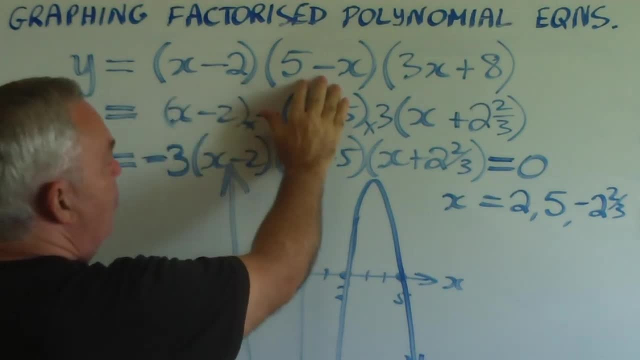 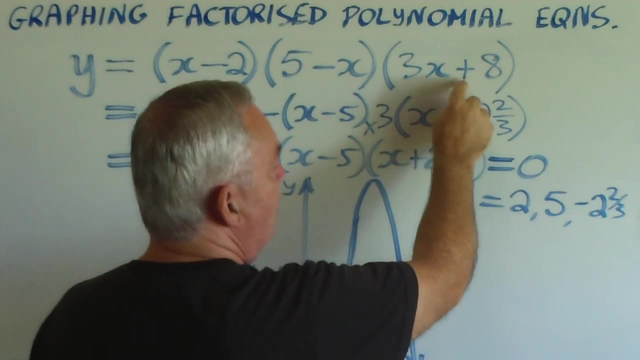 and read that we have a root at 2 and a root at 5, because 5 minus 5 makes 0. If you can calculate quickly, you can see that we have a root at minus 8 over 3, which is minus 2 and 2 thirds. 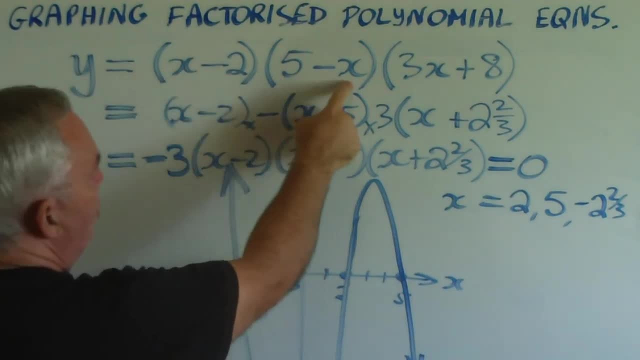 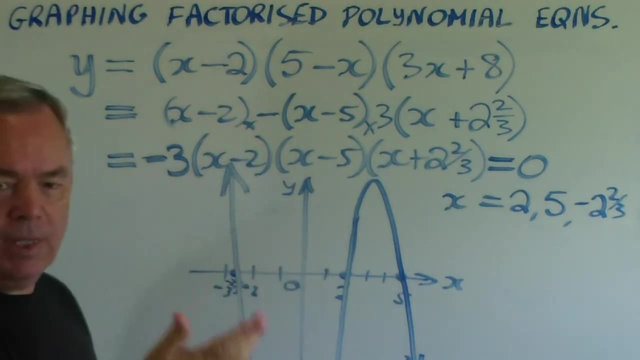 And then, if you check the leading coefficient by looking at your x values, we can multiply 1 by minus, 1 by 3, which gives us a minus 3 and an understanding of what's going on. So you need not do all these calculations.